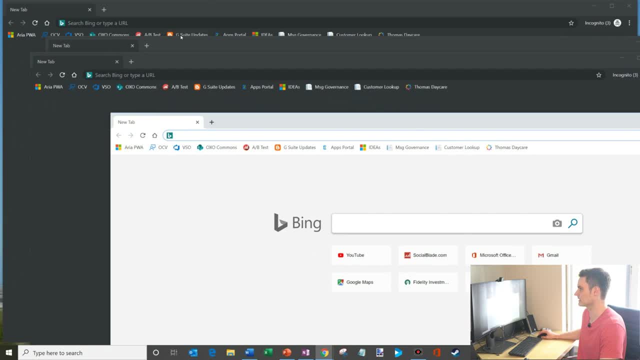 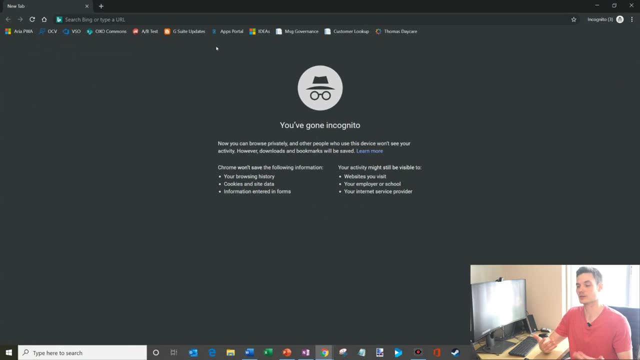 that also opens up an incognito window. So here I have, all these private browsing sessions Now that I have the window up. I just want to talk about a few things about the window, though, and some things that you should be aware of, So you'll see these little bullet points on the page I'm 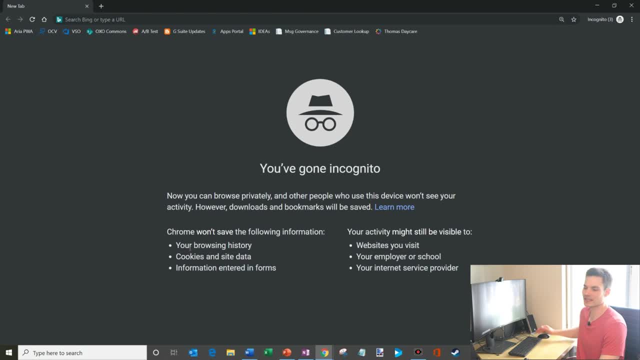 going to zoom in a little bit so we could see that nice and clear. So by being in this private session, what that means is that the browser won't keep track of any of your browsing history. So any websites you go to- let's say you go to Amazon- you're going to see that you have a lot of 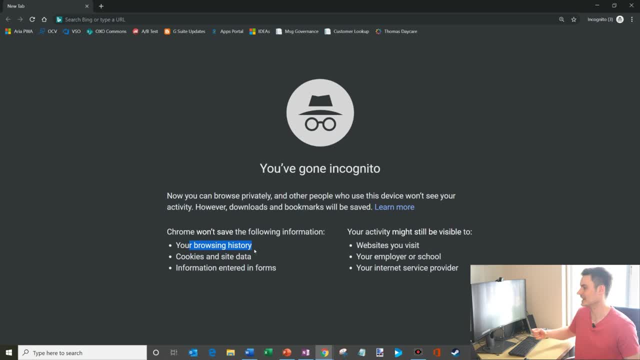 information. So if you go to Amazoncom to buy your mom this gift, it won't keep track of the fact that you went to amazoncom. The browser won't store any cookies or site data, So you won't get any of those. And lastly, if you fill out any forms, let's say you fill in your address, for 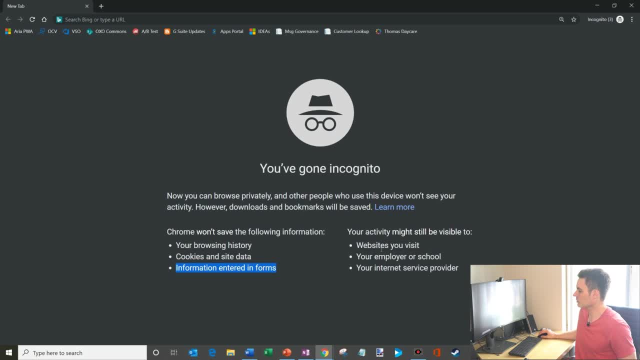 shipping for this gift for your mom. the browser won't keep track of that. What it won't do, however, is if you visit a website, the website will know that you visited that website. If, let's say, you're in school or you work somewhere, they'll probably have tracking where they could see what. 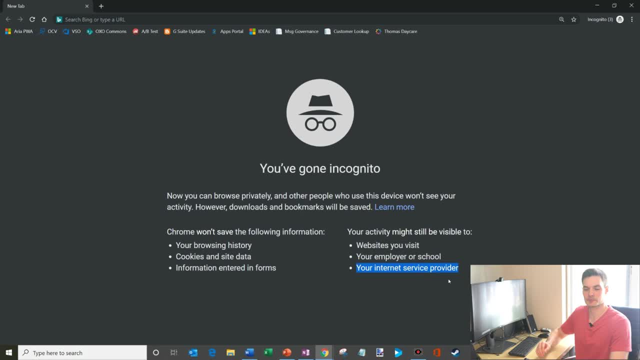 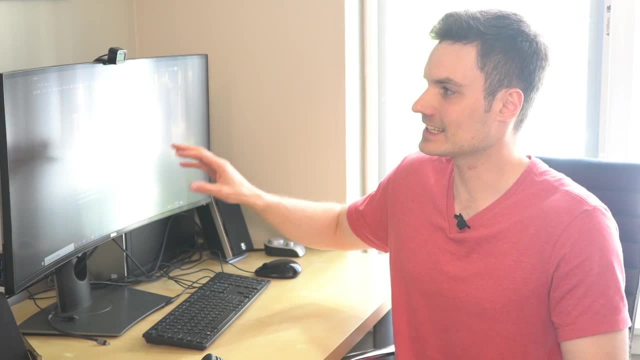 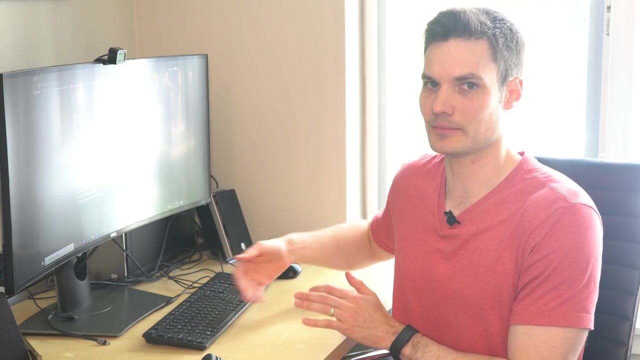 websites you go to And lastly your internet service provider or your ISP. they'll also be able to see what websites you go to. So all that incognito or in private browsing does is it keeps what websites you go to on this device. It keeps that private, but anyone downstream internet 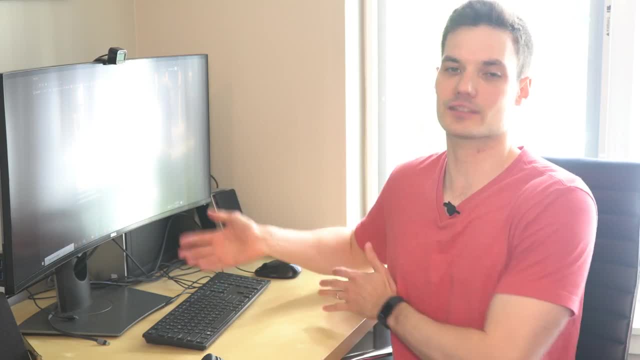 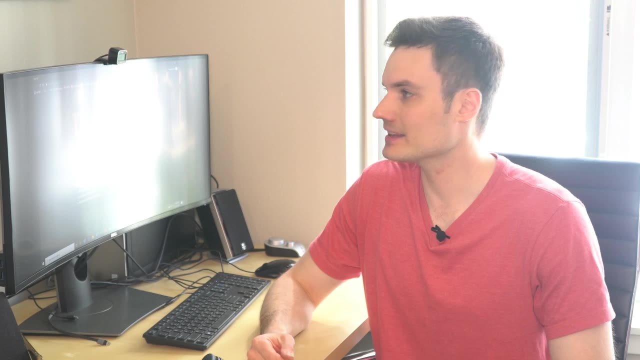 service provider, employer, school websites. they can still see what you're doing on their site, But it's still very beneficial if you don't want people on your machine knowing what you're up to, And that's as simple as it is. 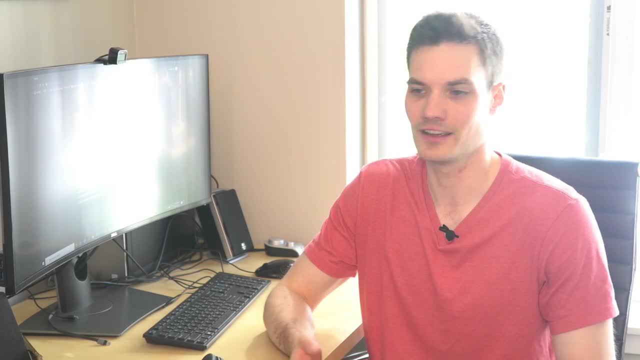 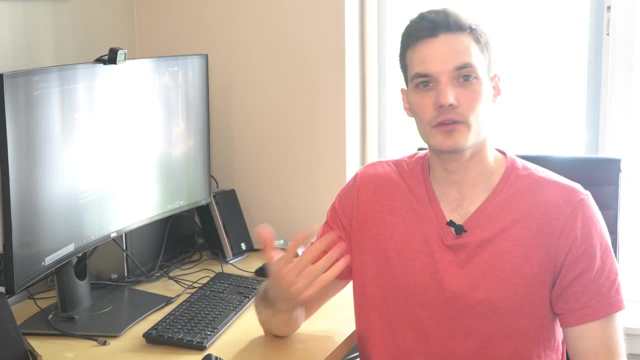 So it's pretty easy to turn on incognito mode or private browsing session- Very simple to do. I showed you three different ways to do it. Hopefully you found this content helpful. If you did, please give it a thumbs up. And if you want to see more how-to videos like this in the future, please hit. 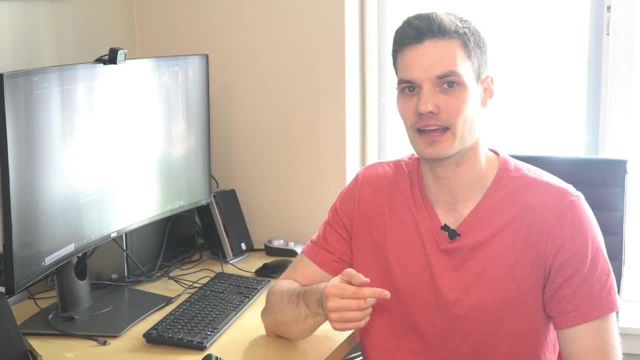 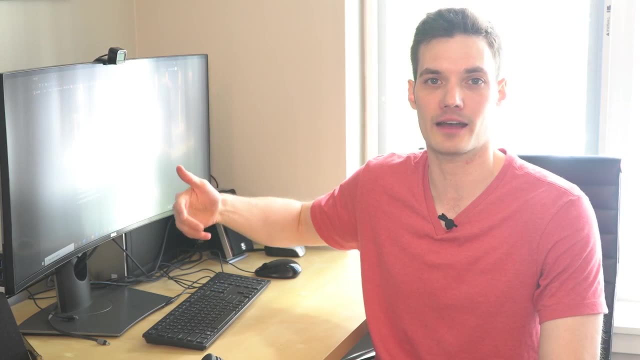 that subscribe button. That way, you'll get a notification anytime new content like this comes out And if you want to see any other video topics in the future, have a nagging question that you want to know how to do. in the comments down below, leave a comment about what you're trying. 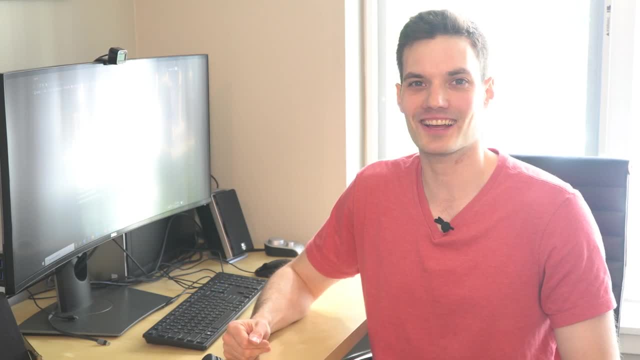 to do And I'll add that to my list of videos to create. All right, Well, thanks a lot. Thanks for watching. See you next time. Bye.